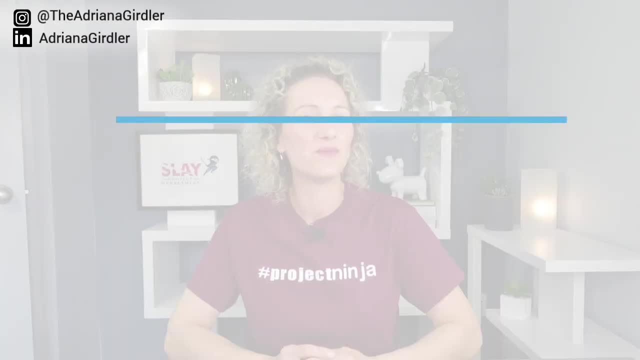 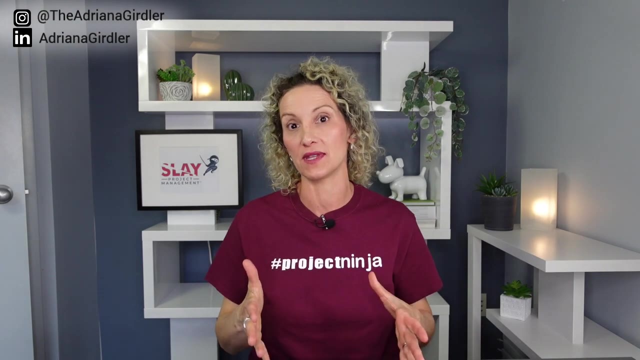 great content And let's get to it. Communication Plan 101.. Okay, what is a project communication plan? It actually is a document that lets you create an awesome project communication plan. It actually is a document that lets you create an awesome project communication plan. It also lays out all the types of communication that you're 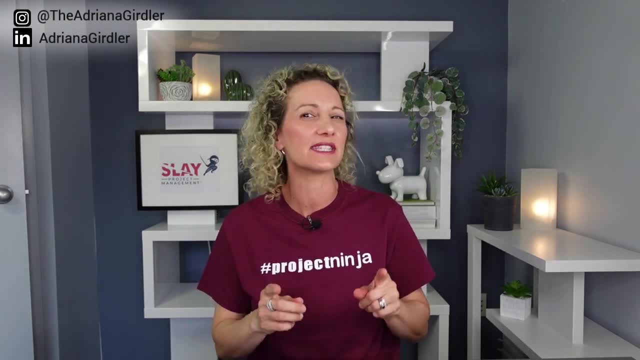 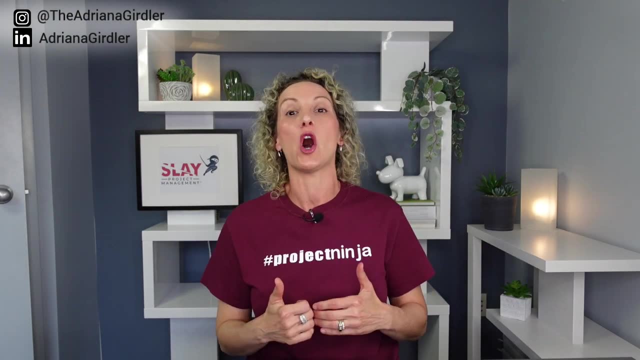 going to have within your project, And it also lays out who are the stakeholders who are going to receive that type of communication. Now, stakeholders, don't forget, range from anyone within your team all the way out to, let's say, senior executives who are just on the peripheral. 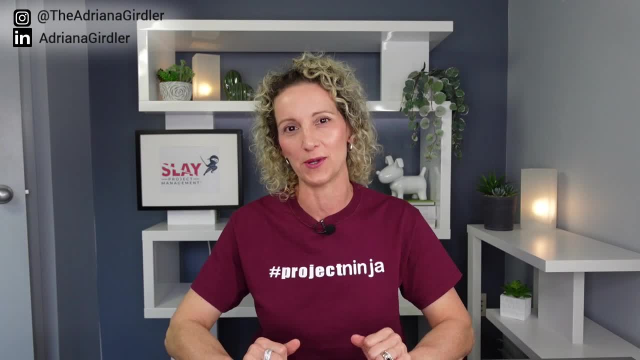 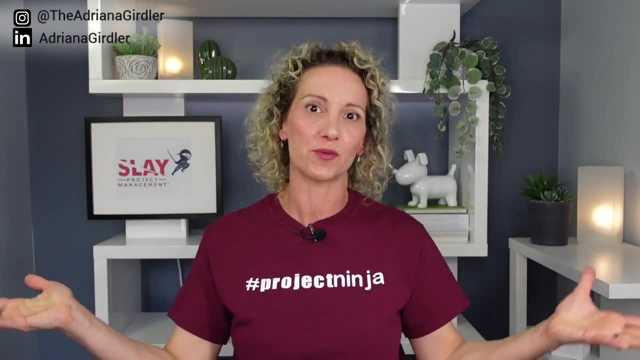 edge. It could also be the end user of that project deliverable. Now, why is this so important? You're probably saying to yourself, Adriana, I am so busy. Seriously, you want me to do a communication plan on top of all the other plans I have to do? The answer is yes, absolutely. You're going to want to. 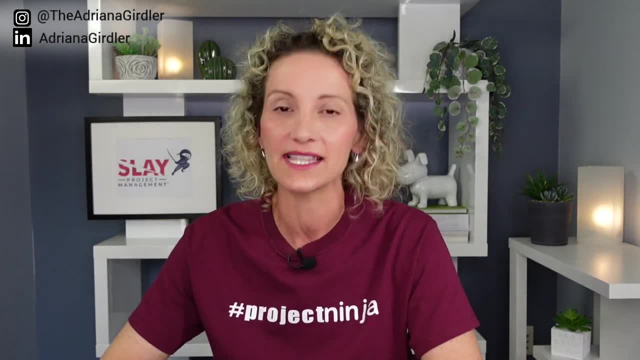 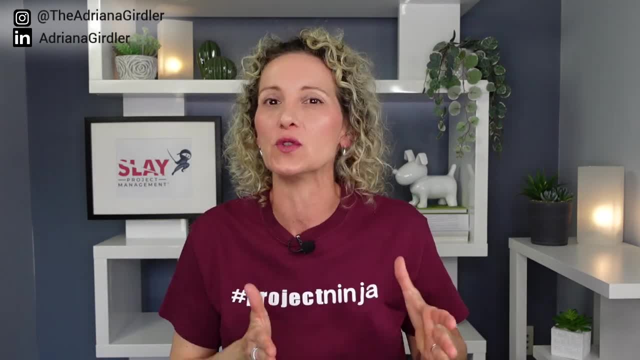 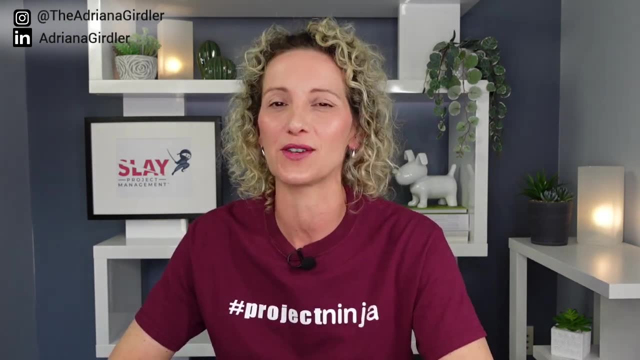 to save you a lot of headaches and heartaches within your project. Now good communication really does equate to good project success. How many times have you been on a project that people assume stuff? It really does hurt the project. So that is why it is so critical for you as a project. 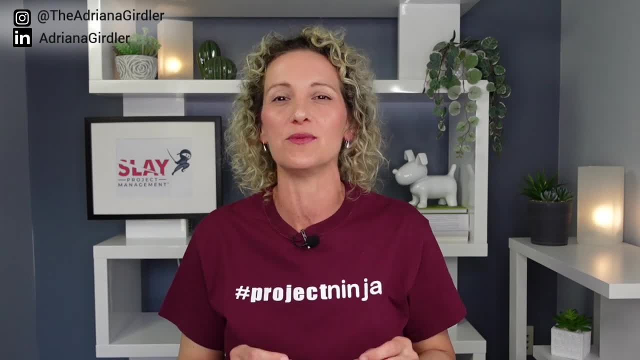 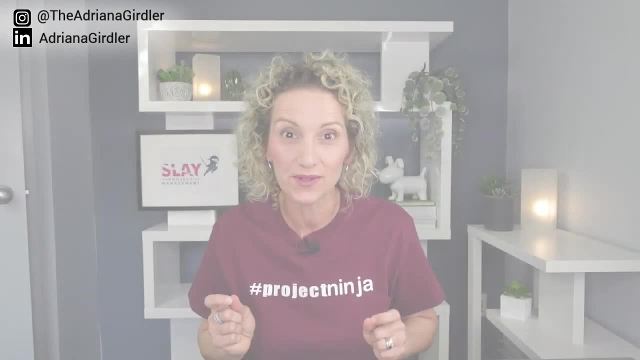 manager or project lead to ensure you have a really good, strong communication plan. What's in a communication plan? Good news for you: I actually have an example for you. you and we're going to walk through it. let's go. so here's your project. 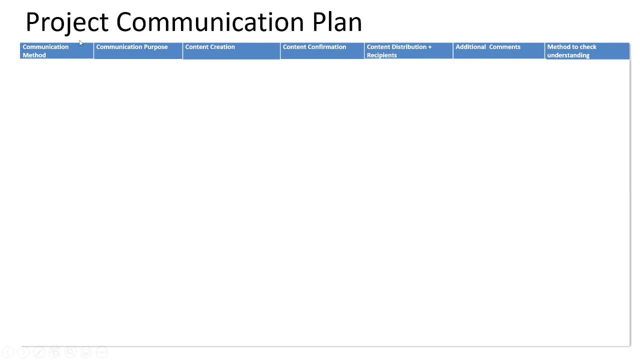 communication plan. it really is a summary document of all the types of communications you are going to be doing within your project during the execution phase of everything. so this is a little summary. it's a matrix. I do mine in a PowerPoint, you can do it in a Word document, whatever it's going to suit. 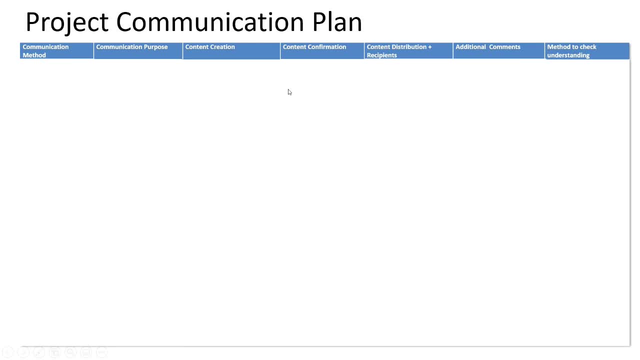 your needs. there's no right or wrong. it really is just summarizing how you're going to do your communication to all of your project stakeholders. so let's talk about each section here so you understand what exactly you do in it. so communication method: this is a type of communication you really have to think. 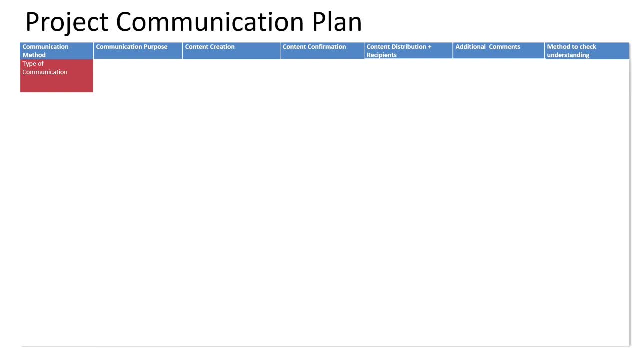 it through. how am I going to communicate with people? and not everybody deserves the same type of communication. you're definitely going to be talking to your project team a lot differently than you're going to be talking to your steering committee, than to senior executives, even to the department or 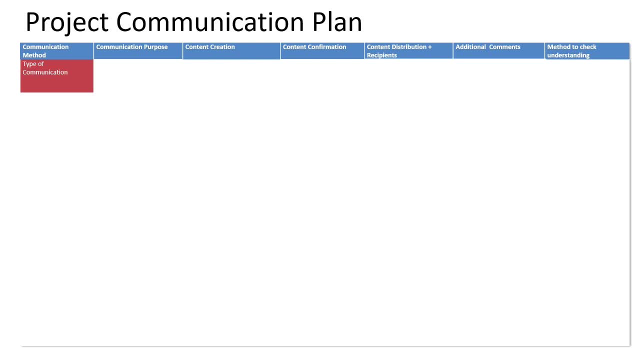 manager who's going to be. you're going to be talking to your steering committee, then to senior executives, even to the department or manager who's going to be receiving your information. sorry, your deliverable and how you're going to communicate to them is so much different. your communication purpose is: why is this? 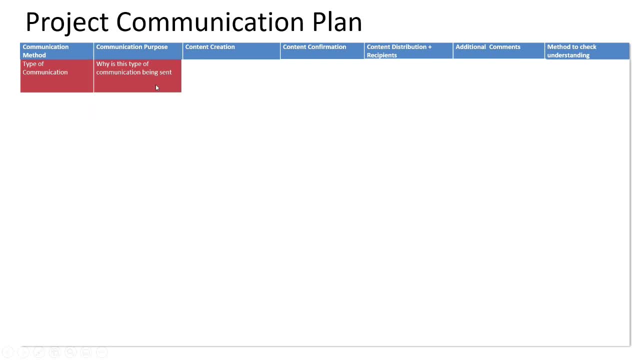 type of communication being sent. you really need to have an understanding of this, as this is going to help you understand a whole bunch of other aspects like content and frequency and stuff like that. you're going to also say who's going to create the content, so this is content creation. a lot of times, 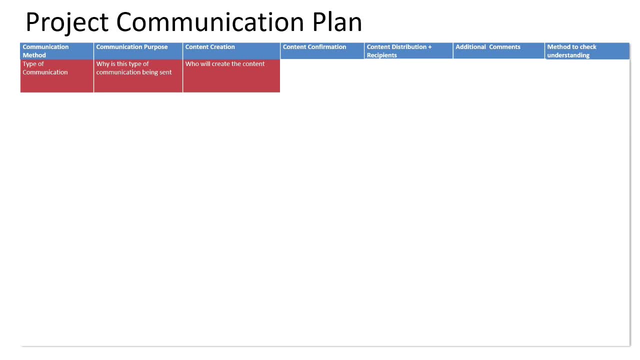 when it comes to communication, it usually falls on the shoulders of the project manager, but sometimes it has to be other individuals. so this is where you're going to really lay it out. content confirmation- who's going to check it? so how do you know that the information has gone out is correct? now? 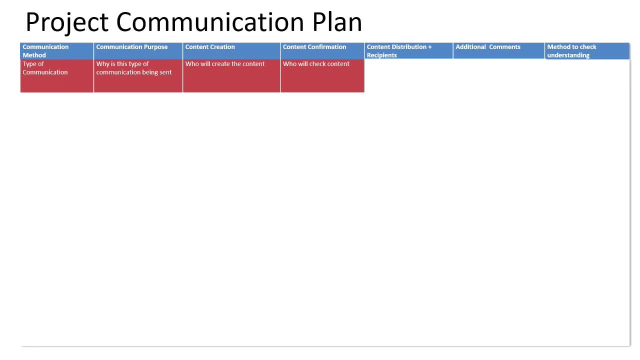 for some instances doesn't matter about content creation because it's staying within the project team and it's not being distributed or disseminated to anybody else. but if it is, you want to make sure that those things are checked and everything is okay from a standpoint of acceptability from communication. 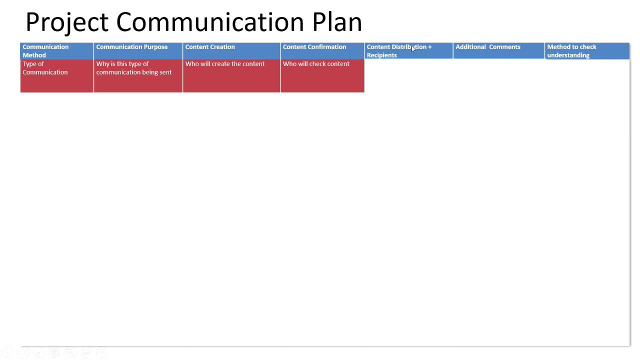 standards, company standards, things like that, things of that nature- content, distribution and recipients. so who's going to send it out and who will receive it? again, not all communication is going to be sent from the same individual. I may have an announcement that I created and that I need the president of the organization to send on. 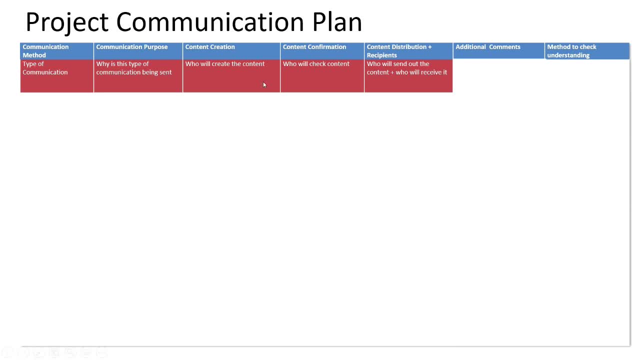 my behalf from a project communication standpoint, if I want to give some like an announcement to an organization of what's going on again, it really is dependent on your type of communication. additional comments. so you, those are your attachment, who needs to be cc'd and method to check. 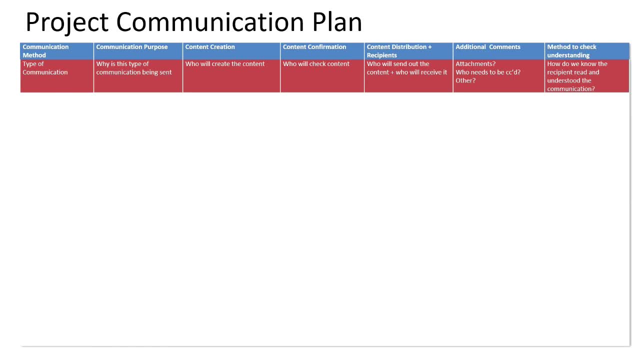 understanding. how do you know that your communication was read and understood? this does not have to be detailed. this not does not have to be complex. just a simple outline summary sheet can make a huge world of a difference as to how successful you're going to be with your project. because I've said this before: 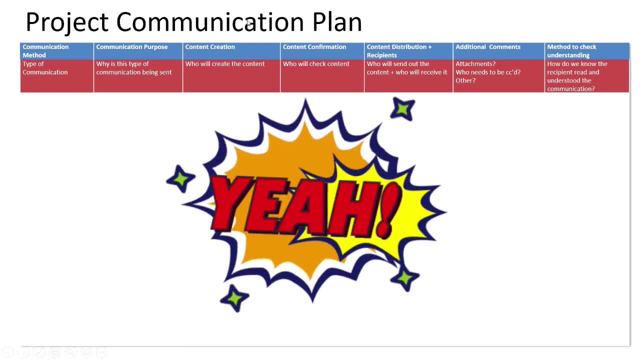 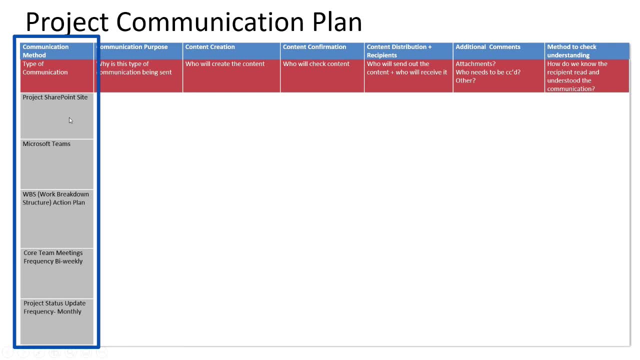 communication is the heartbeat to a really good, successful project. so now what I want to show you is I want to share with you some types of communication. this is not an exhaustive list- all right, it's not. it's just an example so you can have an understanding as to what are some of the things. so 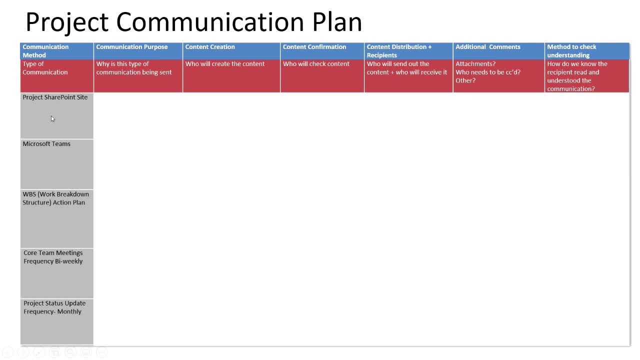 let's look at some of this in a little bit more detail. so we have a project SharePoint site, Microsoft teams, we have a work breakdown structure, an action plan, we have core team meetings, project status update- so you can have a lot more stuff. in here you can actually lay out every type of 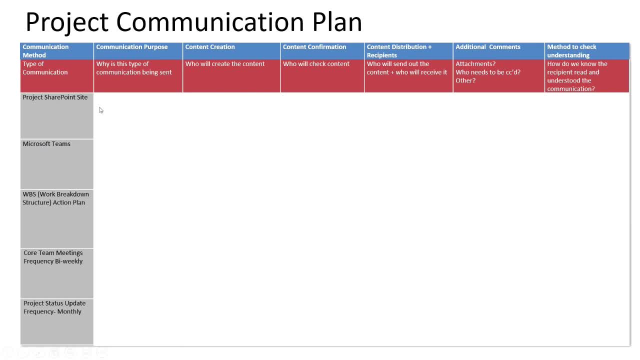 meeting you're going to have, you can actually lay out some- even change- management aspects as to how are you going to make announcements to end users, depending on what your project is. but again, for sake of simplicity, I just want to share with you a few so I can explain how you fill the rest out. so let's take. 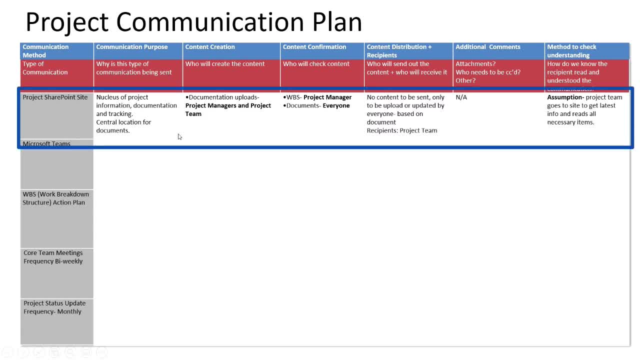 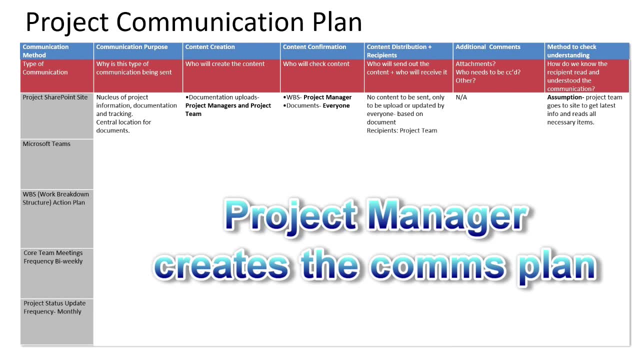 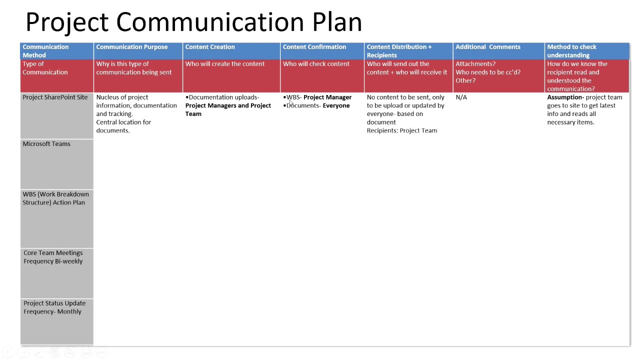 a look at project SharePoint site and go into a little more detail, because, again, I do mine in a PowerPoint, I slip it into my charter and, as a project manager, this is my job: to decide how is communication going to be unfolding in this project, and there may be some instances where you want to bring in your team to ask them for some. 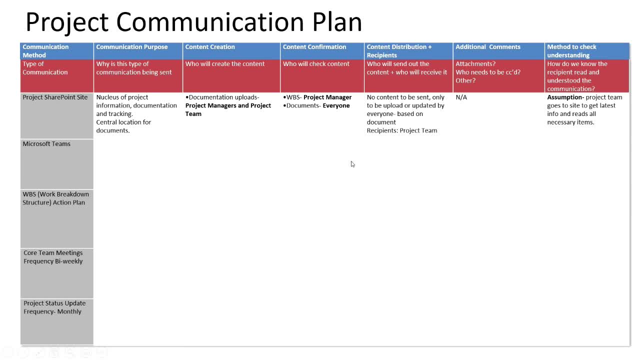 feedback, particularly if you're going into a lot of in-depth change management aspects, which are talking about end users and the communication and training that you need for them. but if you take my slave project management course, which I put the link underneath this video, I actually talk about all of that in great detail, so I'm not going to go into. 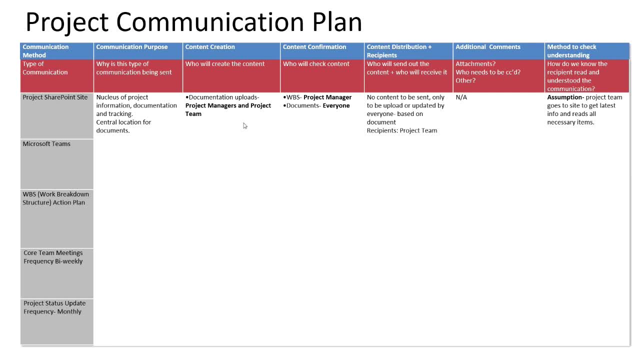 it here. so if you want more information, definitely check out that link. so let's talk about this project: SharePoint site. I'm a big believer in having a central location, and for us, why is this communication even being done? because it is the central place of our project. it's where we have all our documentation. we 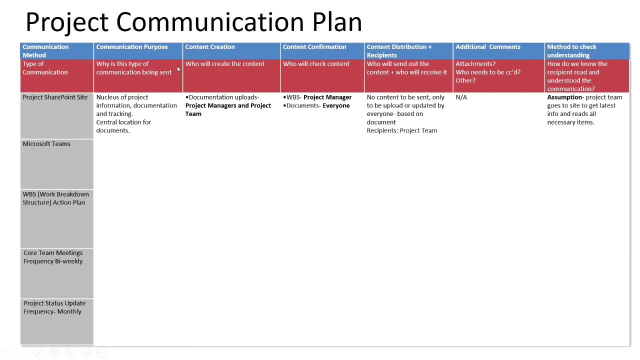 track everything we even communicate in it. and so who's gonna create this content for the SharePoint site? well, this document uploads and it's the manager, the project manager and the project team who's gonna do this and who's gonna check the content. well, WBS, which is my action plan, I check that. 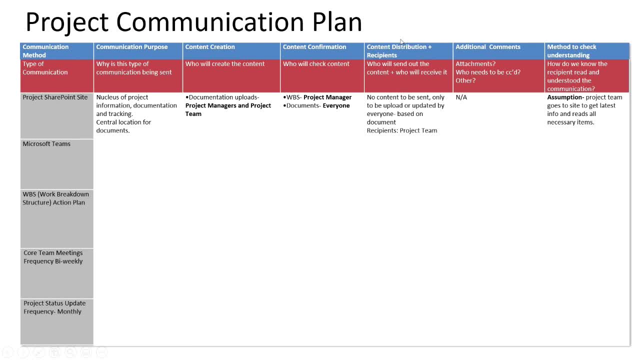 content and for documents everybody else does. now, under content distribution and recipients, there's no content to be sent, only uploaded and updated by everybody, and that the recipients is just the project team. remember what I said earlier: every single part or every single piece of communication doesn't. 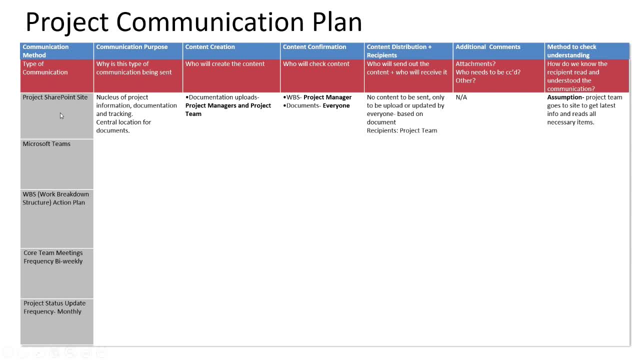 necessarily have to be distributed to the project manager and the project team so you can have specific pieces or types of communications for specific stakeholders. that's absolutely acceptable. and then we're not having any attachments. and how do we know that everyone read and understood? is we're? 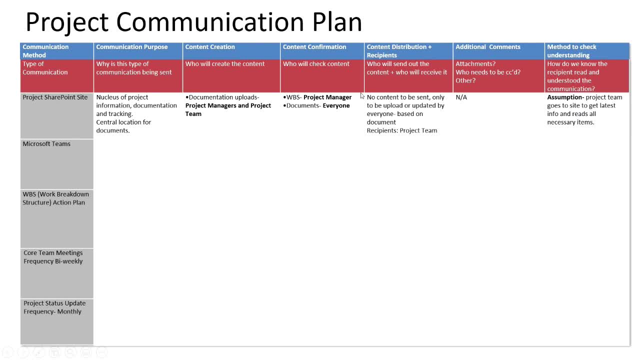 having an assumption that people are actually following our ways of working. so that's one type of communication method. it's not your traditional communication method, but it definitely is. how this project is communicating is we're really using it as a point of reference and information. so let's talk about Microsoft teams, this here. if we take a 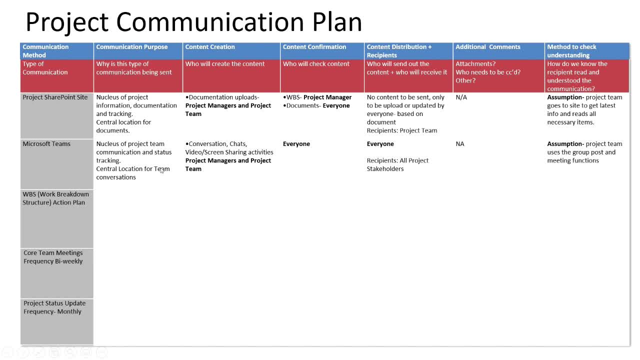 look over at this column is for every single stakeholder. this is where we're communicating and we're tracking status and we're having conversations and video screen sharing, and we're doing this to keep everyone in the loop, so everyone can have the ability to do it. no one necessarily has to manage it. it's the 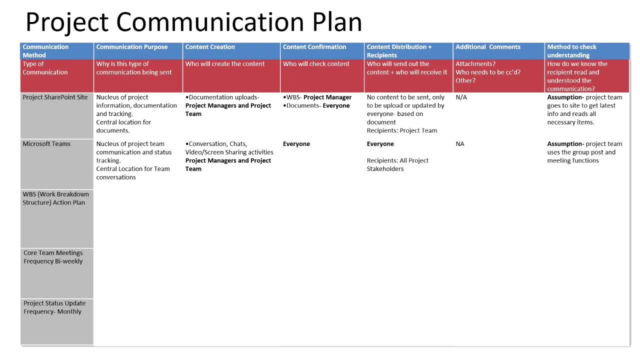 conversation you start in the posts and with chats, and it's a lovely way to ensure that everyone is able to do it, and it's a lovely way to ensure that everyone is really kept in the loop in real time. so that's something else we're doing as a project as part of our project communication plan. now your 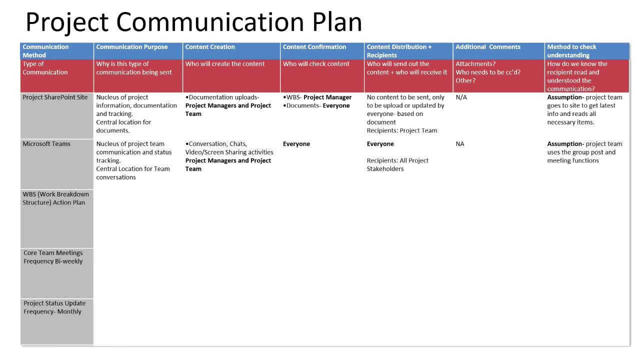 action plan. some people may not think to put the action plan because a lot of times when we think of communication plans, we're thinking outside of our project team. we're thinking of the end users and, yes, you can definitely do this. what I'm showing you here really is more of internal project communication ways. 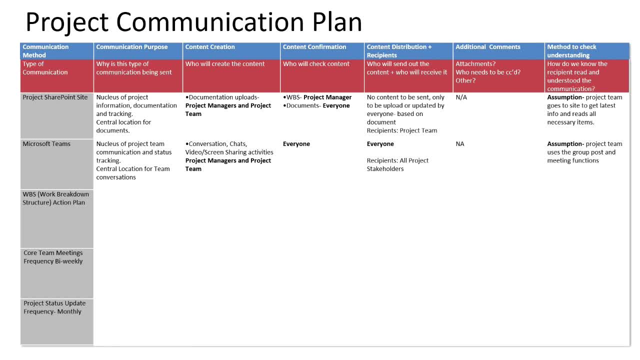 of working, but it's just as important as our external ones, which is usually like to the end user or the individual department who is receiving the deliverable. so why do I put my action plan here? well, as I said before, I have a course like project management and I use a WBS very heavily. 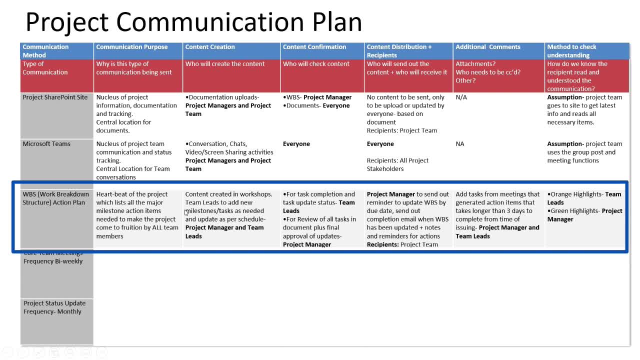 it is the heartbeat of the project and I not only use it to track tasks, but I use it to communicate as well on status. I do not hold status update meetings. we actually use a WBS to be monitoring. all of that- and that's why this is part of our communication- is because we have to have 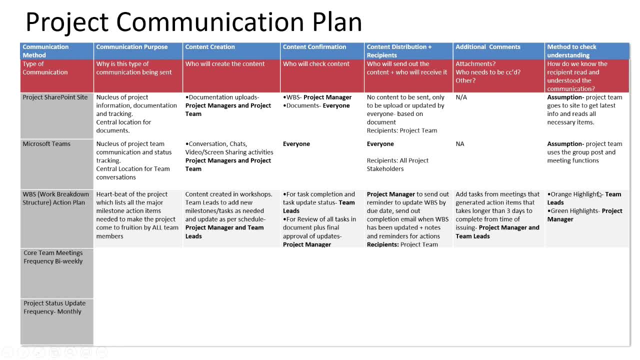 an idea as to how we are going to go about using it, and we use it with a color coding system and a comment column where, based on those tasks, updates can be given. I can question, I can ask questions and then mark my comments in green so that my team now knows that I've just spoken to them, and vice versa. 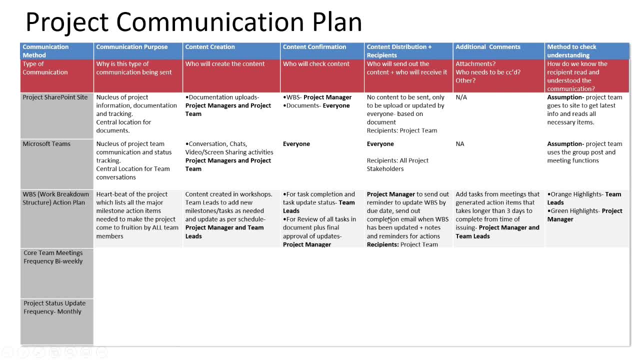 they can speak to me by making their comments orange, and it really is an amazing tool and a simple tool. actually don't need software or anything like that, just Excel spreadsheet that everyone can utilize and use and be involved with. it's a really great accountability tool, but it is part of my project communication. we have core team. 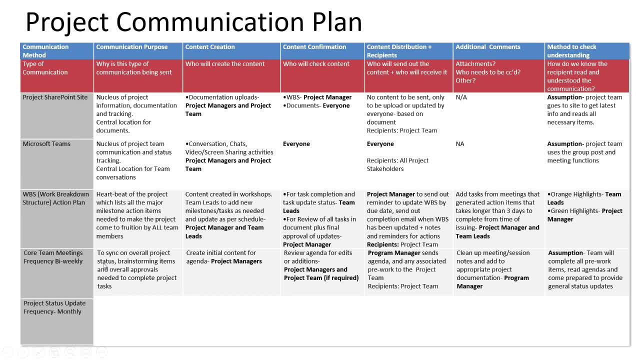 meetings. now you can have as many meetings as you want here, but you can see exactly who I've included in on the meetings, the expectations of them and, just for the last example I want to show you is project status updates: frequency, monthly. so this again, if you take a look at our 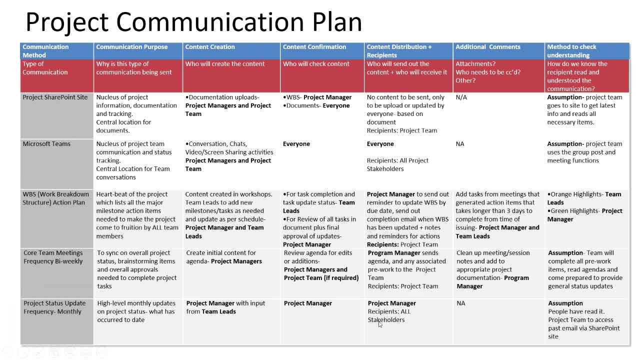 content distribution column and recipients. every stakeholder can get this. I'm the one as a project manager is creating the content with some of my team leads. I'm confirming it. we're giving them monthly updates and I am assuming people have read it. I'm not going to follow up with them in it, but 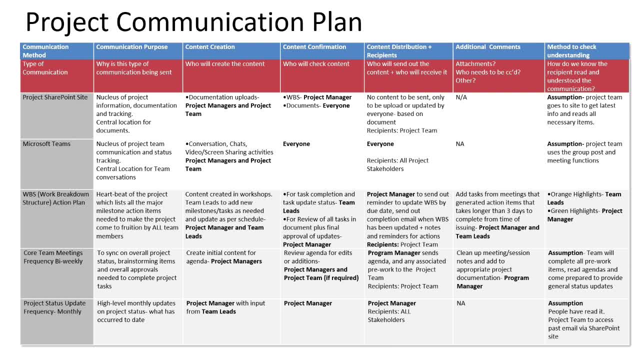 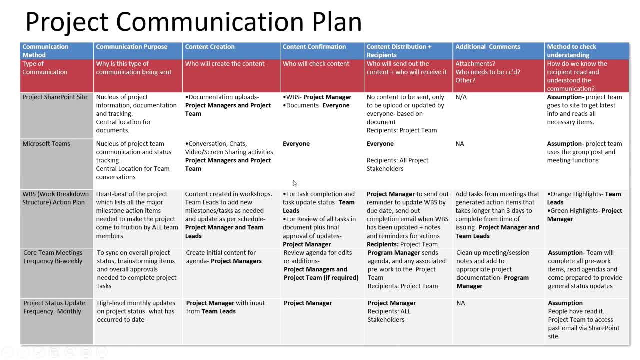 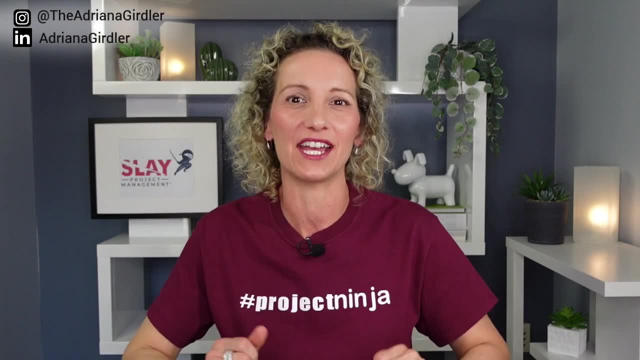 simple, very straightforward. do you, as a project management manager, create this? but it's so worthwhile because it lets everybody know how things are going to unfold, how to use your communication plan. like I said in the example, you're going to slip it into your charter and you're going to present it at your 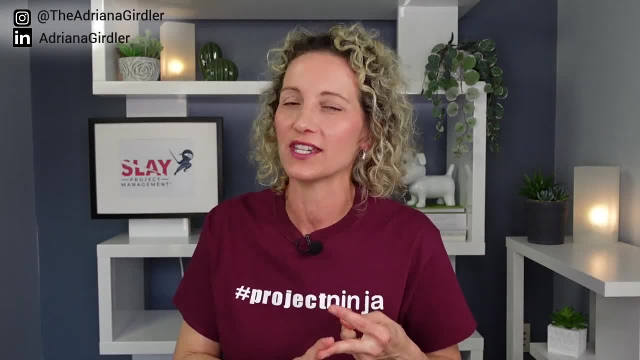 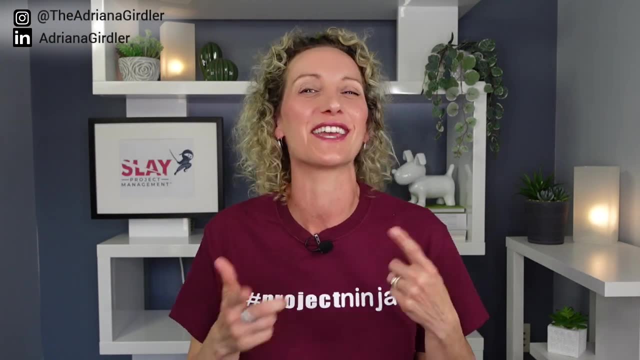 project kickoff meeting now. if you want more information on charters and project kickoff meetings, just go to youtube search Adriana Girdler project kickoff, because I have a video specifically on that, or Adriana Girdler charters, because I have a video on that now. 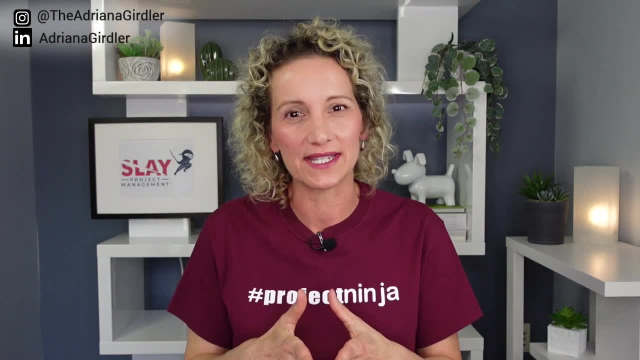 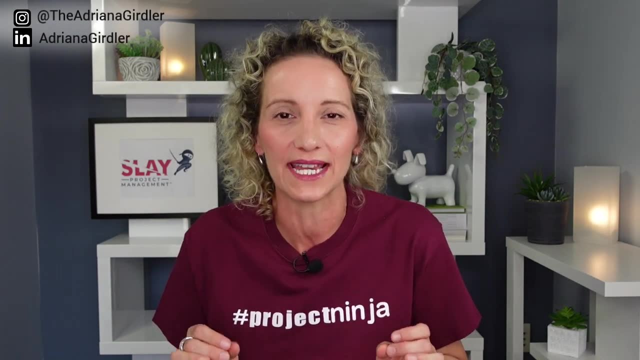 it's really imperative that by doing it at this point in time, you're basically setting everything up from scratch and actually that's at the start. in a very positive way. you're communicating already, you can set up all your meetings, you can already direct people to the SharePoint site- all of that.